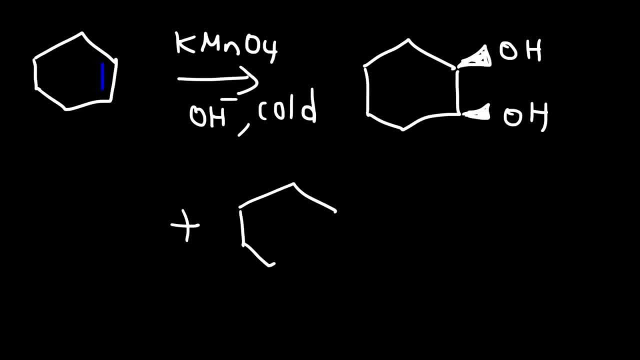 So you can draw your product like that, or you can draw it like this. Now notice that these two products are identical Due to an internal plane of symmetry. these two products are mesoproducts. So therefore, because Because they're identical, we only get one product in this reaction. 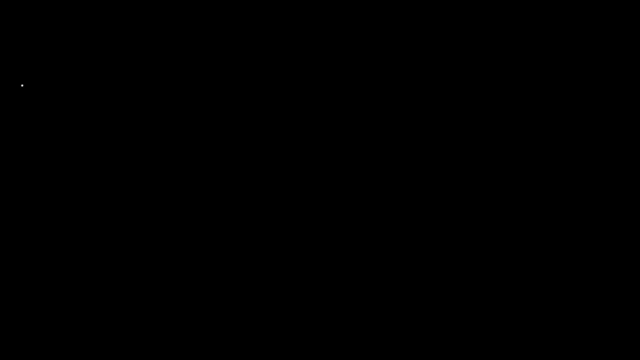 Now, another reagent that can do the same thing is this one, OSO4,, followed by, in the second step, sodium bisulfite. So this will lead to the same product, and that is the cis-1,2-diol. 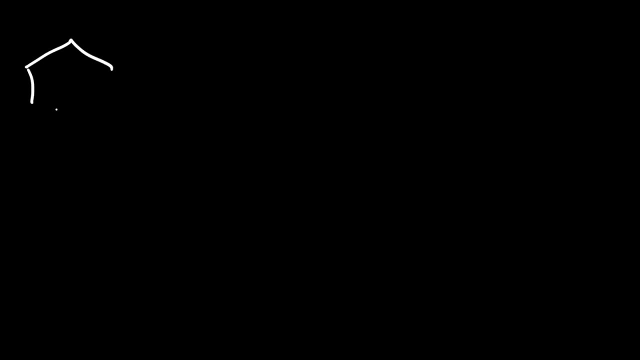 Now let's go back to this reaction. So once we have this alkene and once we react it with potassium permanganate under basic conditions, before we get our final product, we get a manganate ester which looks something like this: 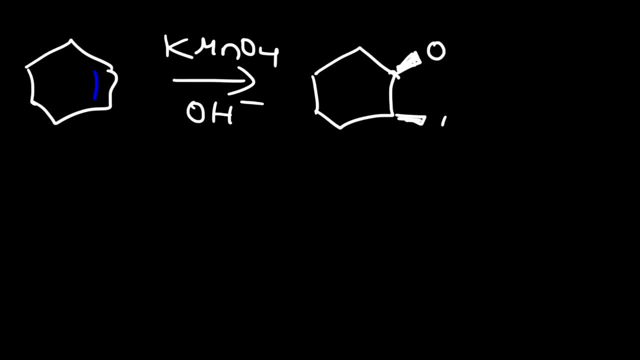 This. But before we get it, here's the reaction mechanism for that step. So this reacts with the permanganate ion, which looks like this: So this double bond is going to break, It's going to connect between these two atoms. 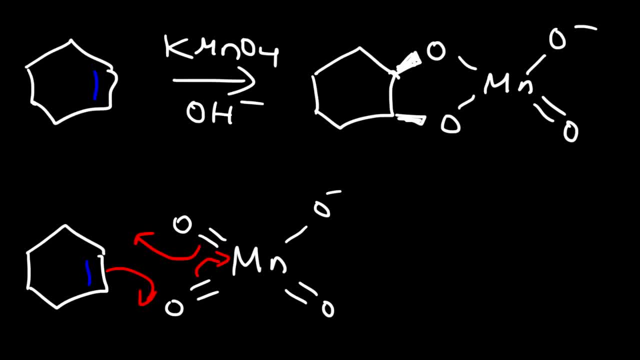 And then this bond will break and these electrons will go back to the manganese atom, And so you should really get this structure, which I don't need to draw it again. So you're going to get this manganate ester, But there should be a lone pair here, so let's go ahead and put that. 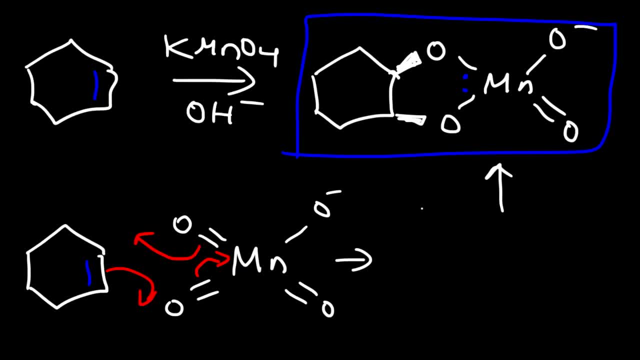 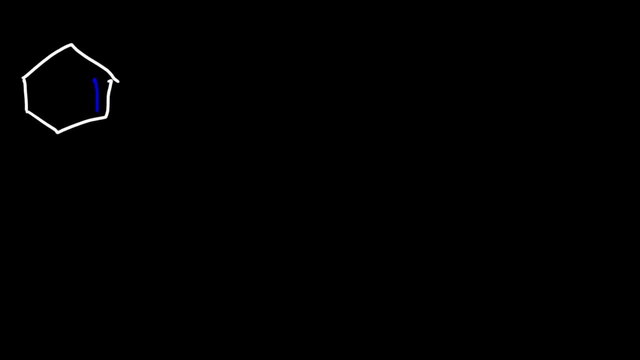 So that's the product of the first step, And then, once you react it with hydroxide- let's go this way- it will hydrolyze into the cis-diol. Now let's go back to cyclohexene And let's react it with osmium tetroxide, which looks like this: 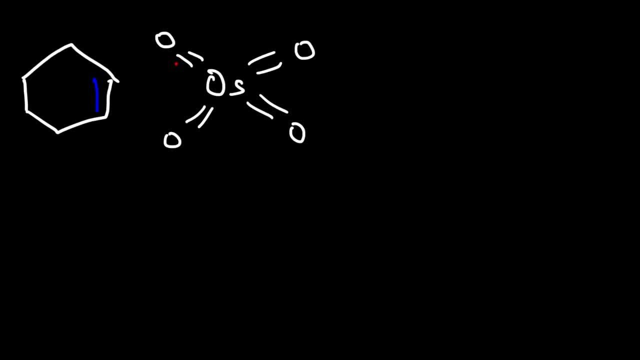 And so what's going to happen is the double bond between the osmium and the oxygen atom will break, and the carbon-carbon double bond will break, And this will give us something called an osmium ester. And so you can see that this mechanism is very similar to the formation of the manganese ester. 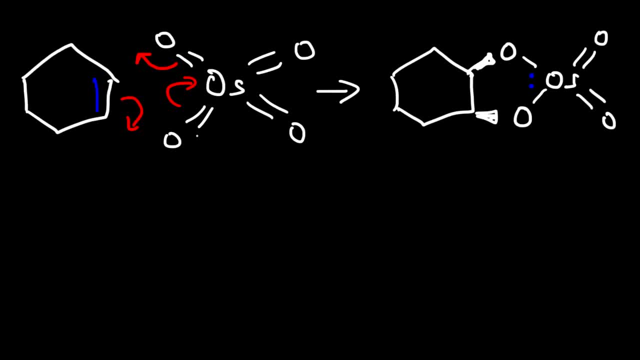 Now we should have a lone pair here. So after adding osmium tetroxide, the next step is to react it with sodium bisulfite, typically in water as well, And the end result will be the same- is that we're going to get the cis-diol. 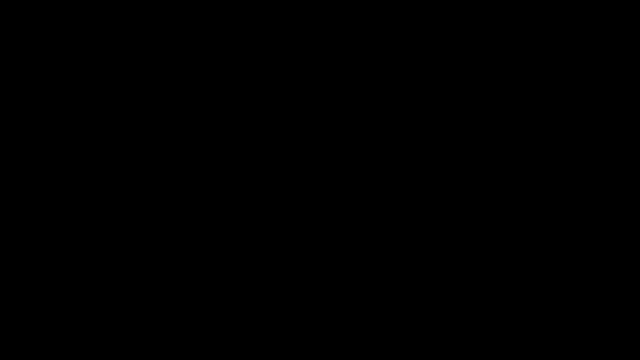 And so I want you to see the step-by-step process for that reaction, Now starting with the 1,2-diol. what do you think is going to happen if we react this with per-iodic acid? Now, whenever you react a 1,2-diol with per-iodic acid, 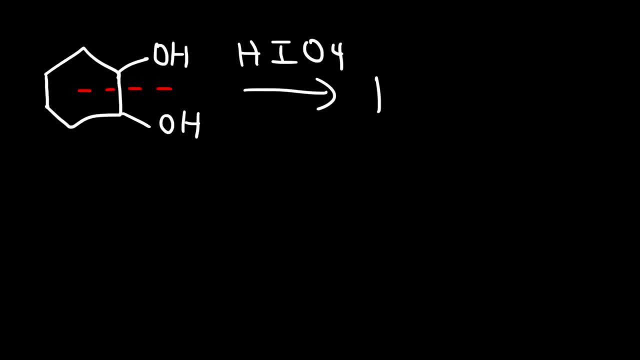 the carbon-carbon bond will cleave, And those 2 diols? they're going to be oxidized into an aldehyde. So you can redraw the structure like this: We have a total of 6 carbon atoms with an aldehyde at the end. 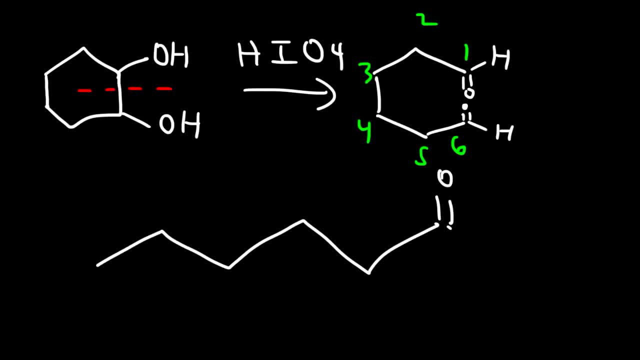 So 2,, 3,, 4,, 5,, 6.. And so this is going to be the product of this reaction. So per-iodic acid can convert diols into aldehydes and ketones, If there was a carbon here. 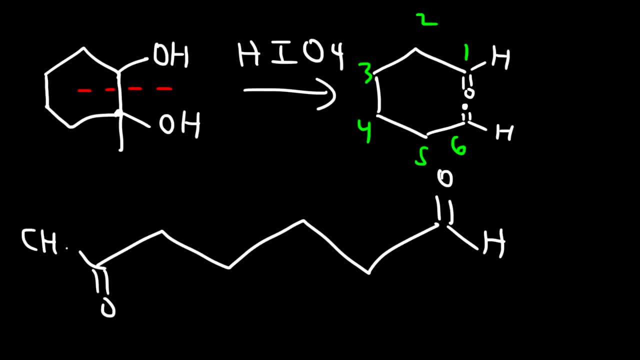 then instead of having, let's say, an aldehyde, this would be a ketone now, But since we don't have that carbon, these 2 are aldehydes. Consider this reaction, Let's say, if we have a cyclohexene ring. 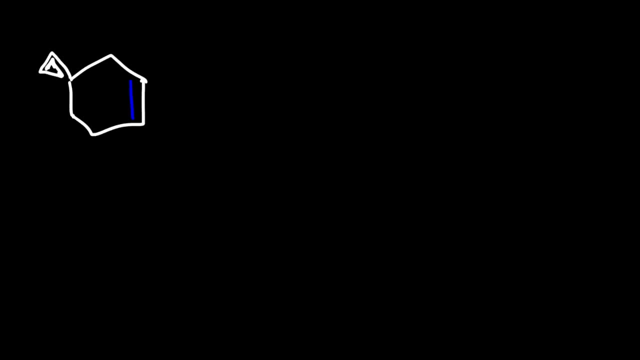 but with a methyl group already present And let's react it with potassium permanganate under cold basic conditions. So how many products will we get in this reaction? So we know we're going to get a diol with syn-stereochemistry. 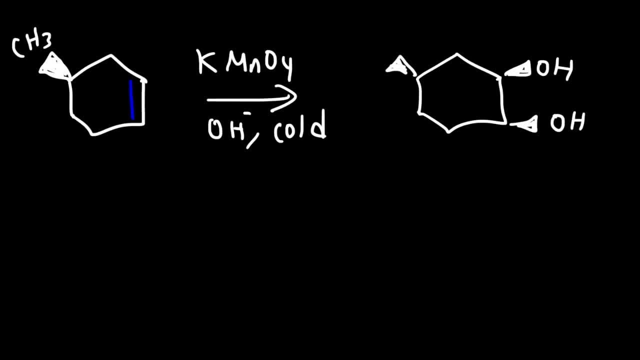 So this is one way in which we can draw the products for this reaction, Or we can draw it this way with the 2 hydroxyl groups on a dash. So what is the relationship between these 2 products? Are they identical or are they different? 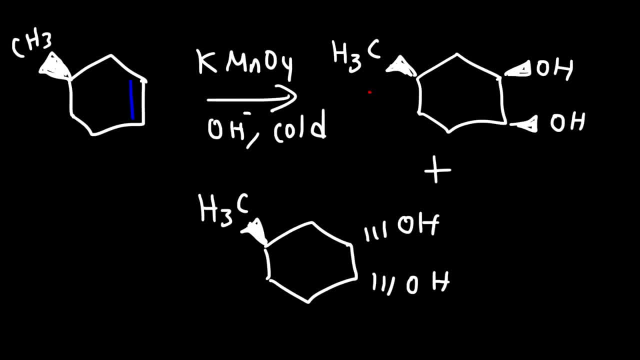 Well, clearly they're different. We don't have mesocompounds anymore. We no longer have an internal plane of symmetry Here. it's symmetrical, but we don't have another methyl group to make it symmetrical across that line. So since we don't have mesocompounds, 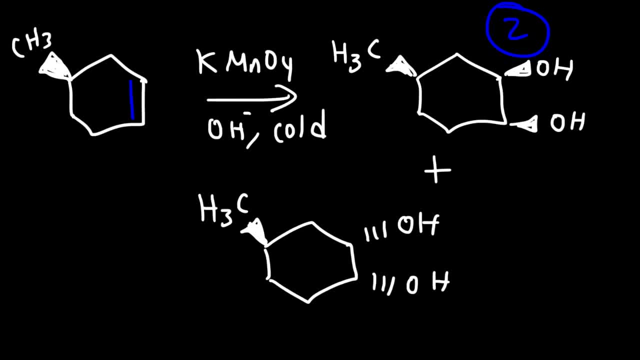 we have 2 different stereoisomers, And would you classify these isomers as constitutional isomers, enantiomers, diastereomers, stereoisomers? What type of isomer do we have? Well, for one thing, these 2 are stereoisomers. 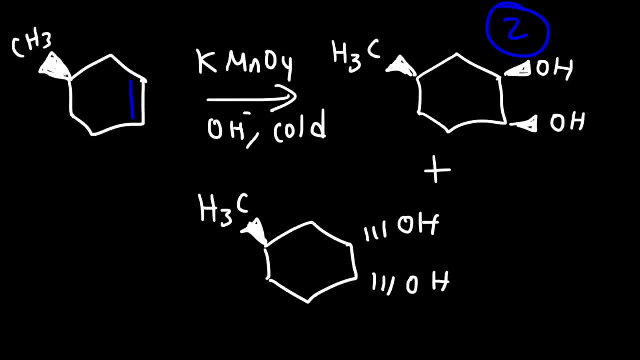 They're not constitutional. Constitutional isomers are isomers that are connected differently. They're connected the same. Let's call this carbon 1.. On carbon 1, we have an OH group, On carbon 2, we have one, And on carbon 4, we have a methyl. 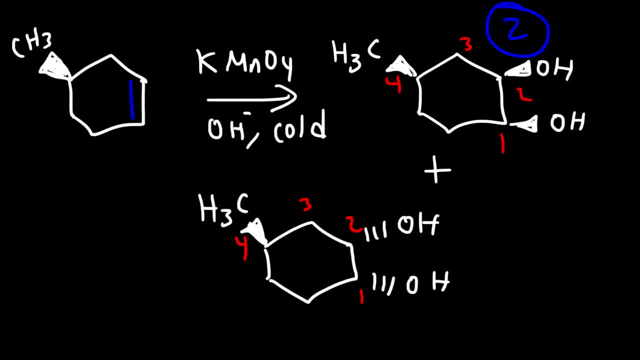 So the connectivity is the same, But the way these 3 substituents are arranged in space is different. So these are stereoisomers. Now, what type of stereoisomers do we have here? Are we dealing with enantiomers, or are we dealing with diastereomers? 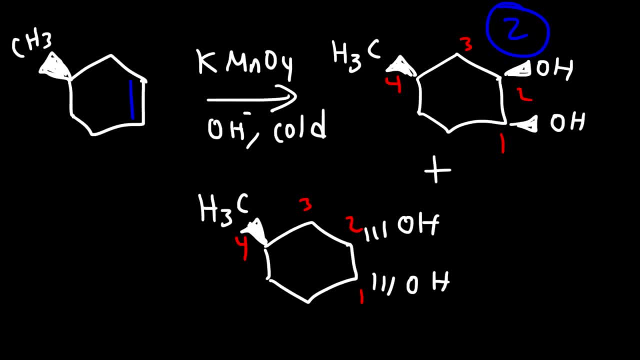 In order for us to have enantiomers, all of the chiral centers have to change. So these 2 chiral centers, they change. They went from being on the dash to the wedge. However, this chiral center did not change. 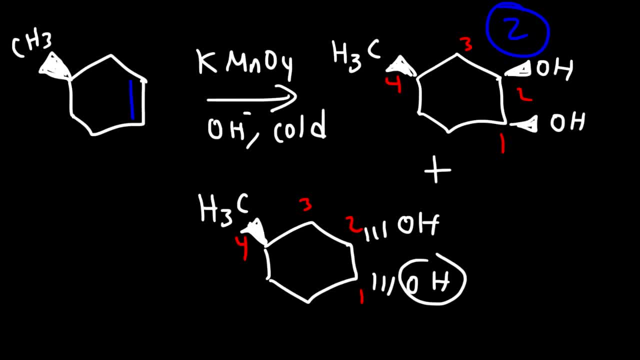 So, therefore, we don't have enantiomers, we have enantiomers. We have a pair of diastereomers. So if some of the chiral centers change, but not all of them, then you have diastereomers. 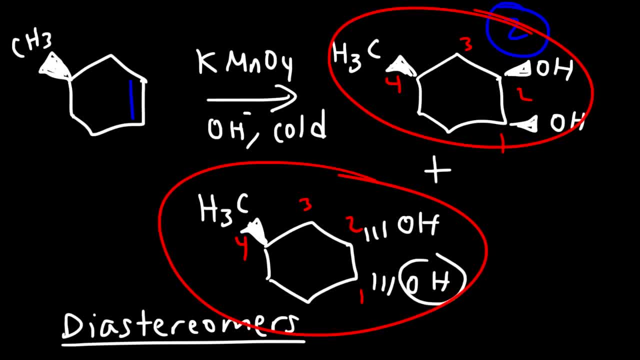 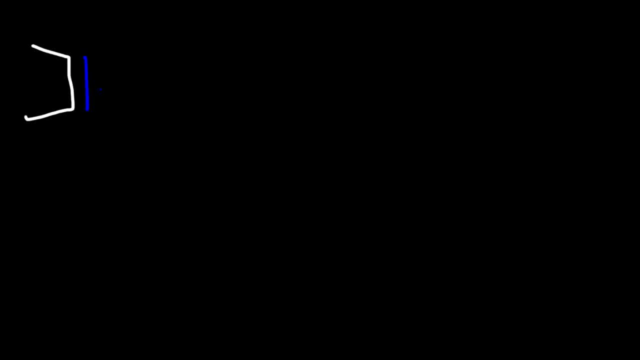 And so that is the relationship between these 2 products. Now let's say, if we have cis-2-butene, What's going to happen if we react it with potassium permanganate, under acidic conditions, with heat as well? Let's say it's concentrated. 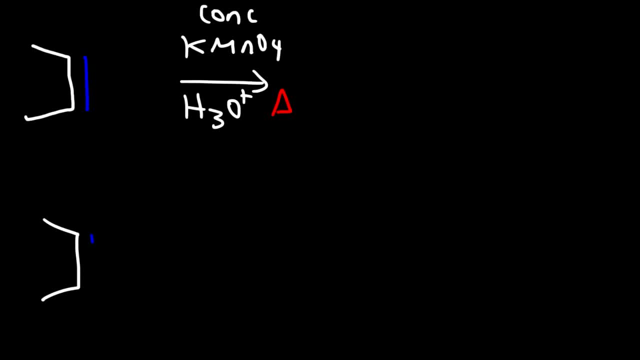 Now let's compare that with cis-2-butene and react in it with potassium permanganate, under cold basic conditions. Well, we know, under cold basic conditions we're going to get 2 hydroxyl groups syn addition. 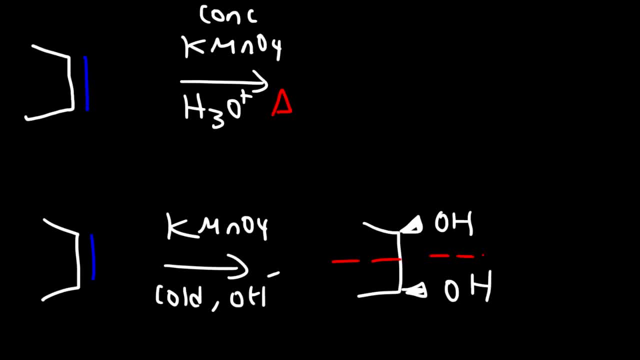 And so this is a meso compound. We're going to get 1 product here. Now, if you, If you use concentrated potassium permanganate, or if you acidify the solution or if you add heat, it's not going to stop at this level. 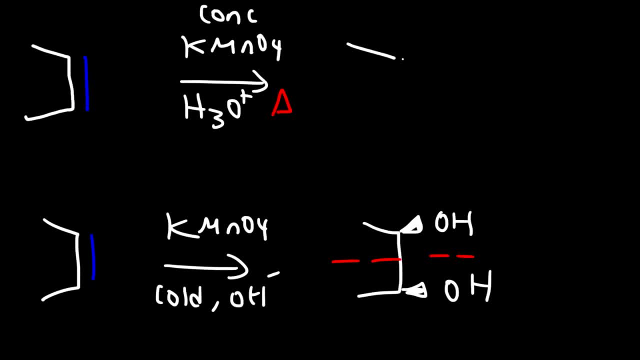 It's going to cleave that carbon-carbon bond, And so what you're going to get is 2 carbosilic acids. If the carbon atom after you cleave it is primary, it's going to be oxidized to a carbosilic acid. 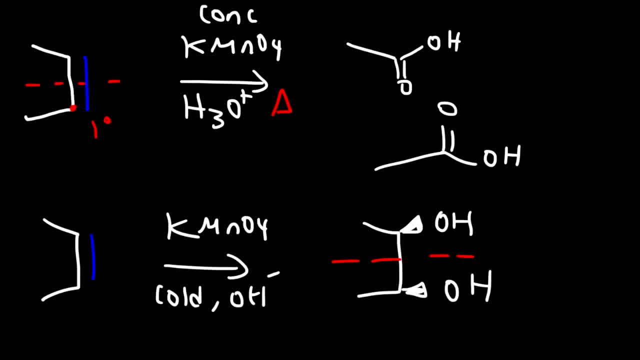 If it's secondary, it's going to go to the ketone level. If it's just a carbon atom, it's going to go to the ketone level. If it's just a methyl carbon, it's going to be fully oxidized to CO2.. 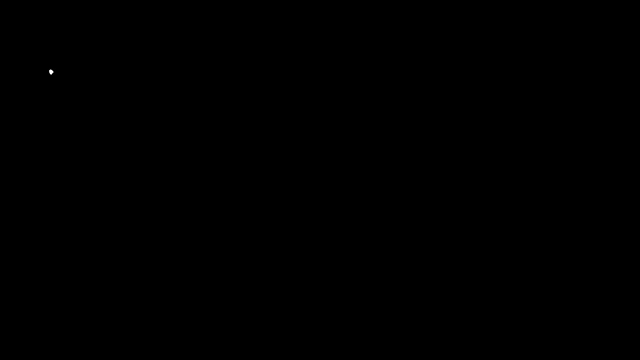 So let me give you some examples. So consider this structure. Let's use potassium permanganate under acidic conditions, So it's going to cleave here. Now what you need to do is separate these 2 molecules And wherever you see a double bond. 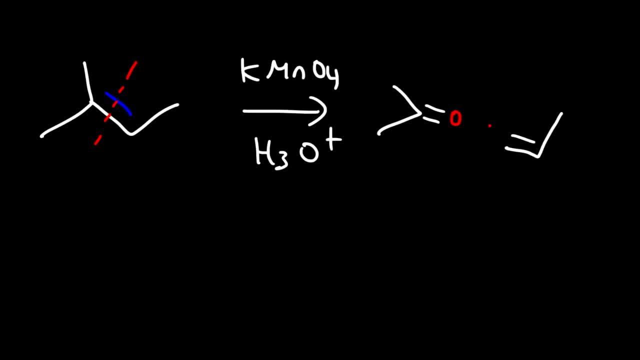 just cleave it, Just add an oxygen to it, And these are going to be the 2 products. So here we have a ketone, but this won't be an aldehyde. It's going to be oxidized to a carbosilic acid. 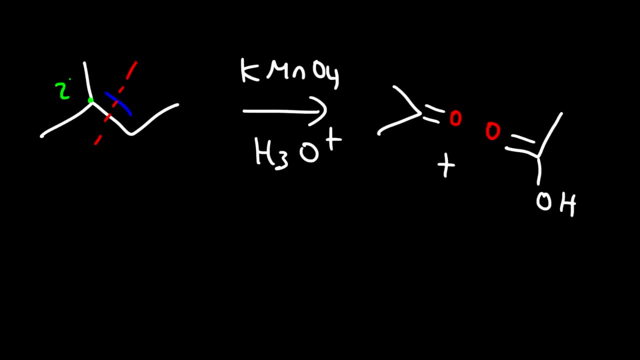 So after you cleave it, this carbon will be secondary, and this will be primary after you cleave it, not before, And so the primary carbon will be fully oxidized to a carbosilic acid. Now here's another example.